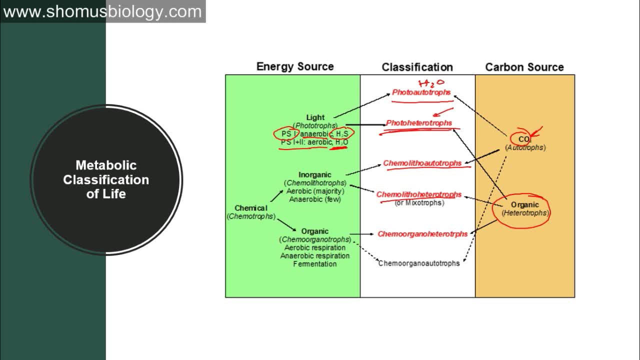 We use the chemical as an energy source, the inorganic chemical as an energy source and carbon dioxide as a carbon source, Chemo, litho, heterotrophs. inorganic chemical as a chemical, so energy source, an organic molecule as a carbon source. So whenever you see chemo, that means the energy sources, chemical. 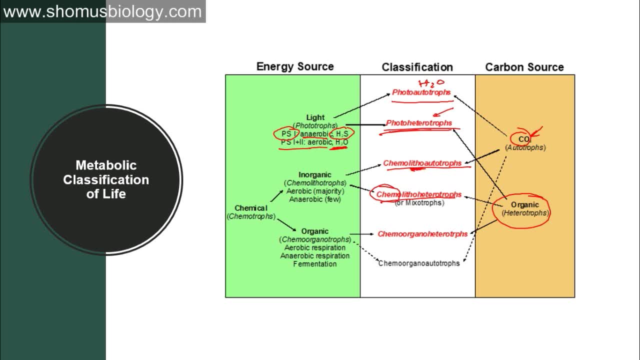 Whenever it is hetero or lethal. whenever it is hetero means utilizing organic compound as a carbon source. whenever it is auto, that means co2 is used as a carbon source. so auto drop means co2 is used as a carbon source. hetero tropics- organic molecules are used as a carbon source. photo trumps light. 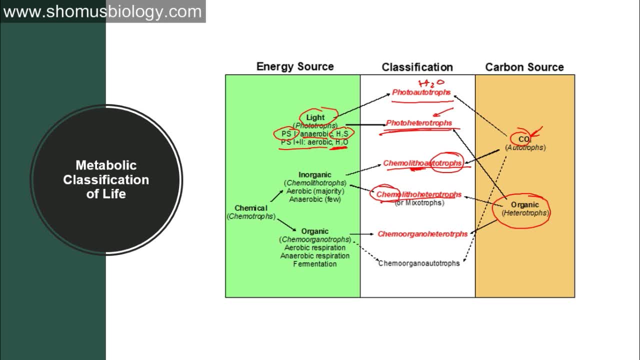 is used as energy source. chemo truck means inorganic or organic compounds are used as carbon source, as an energy source. and last one is chemical, which is organic chemicals, known as chemo organo, heterotrophs, organo. why? because these organic molecules as energy. 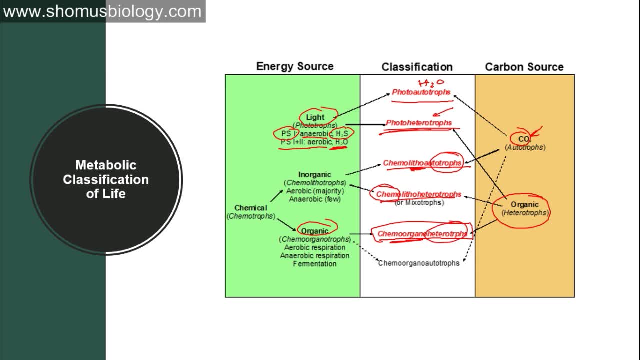 source hetero. why? because they are using organic compound as a carbon source. so, literally, this classification is based on two different source: energy source and carbon source. if light is used, then photo term is used right. if co2 is used as a carbon source, then autotroph is. 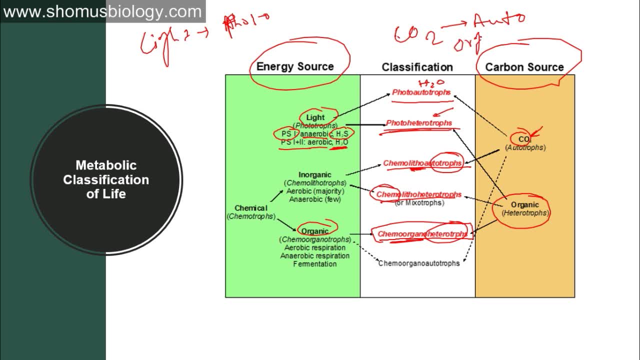 used. if organic molecules is used as a carbon source, then hetero word is used, and if chemical components are used, inorganic chemical used as energy source, then leto is used, and if organic molecule is used as an energy source, then organo word is used. complicated now, but you can easily understand that. you don't need to remember. 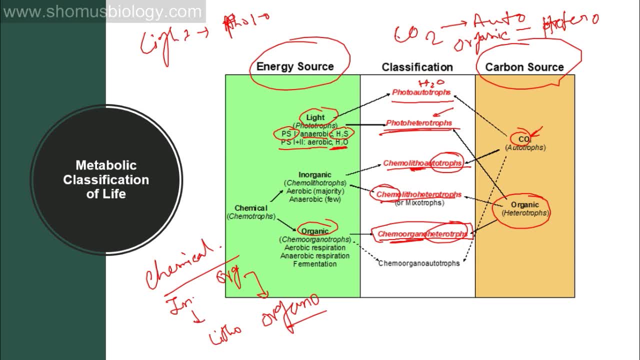 and mug up this. just try to remember: whenever it is used, light uses energy source, than what time is used. when carbon sources co2, what term is used? when carbon sources organic compound, what term is used? And when chemical are used as energy source, then inorganic use, what term is used: organic?